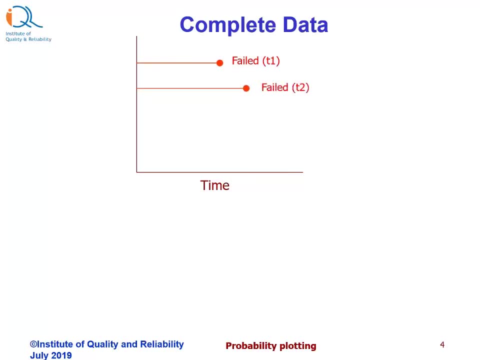 In case of complete data, time to failure of each component is known, ie exact time at which each component fail is known. In this case, the time to failure of all five components is known exactly. The second type of data is right censored data. 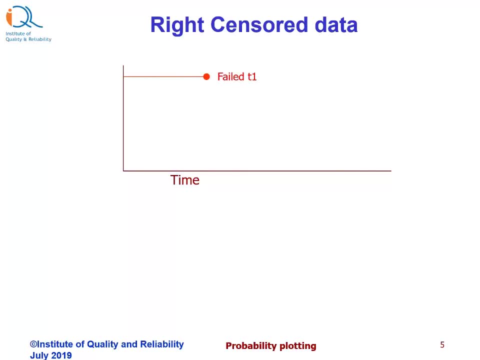 Consider five components here in this case. The first one has failed at time- t1, but the second one is still running at time t2 and therefore we will have to consider this as a right censored data. Third one, also working at time t3 and still running, not yet failed. therefore, this is. 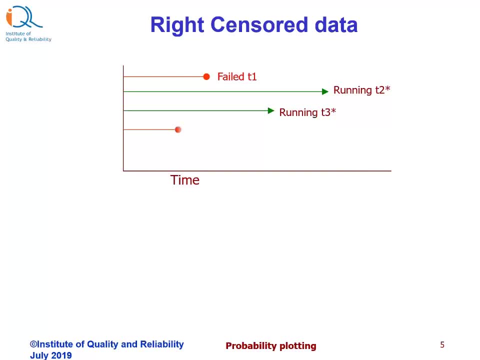 also a right censored data. The remaining two components have failed, So failure times of some units are not known, and this is often the case in the warranty failures of critical items. The right censored data can also occur in case of testing, especially in time terminated. 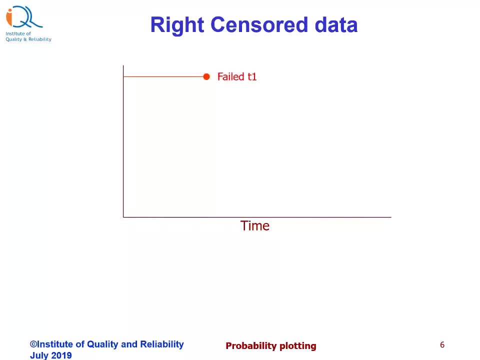 tests Say, for example: we are testing some units. the first one failed at t1, the second one failed at t2.. Third one failed at t3. We continue the test up to time ts until it is stopped. So the remaining three component continue the test up to time ts and have not yet failed. 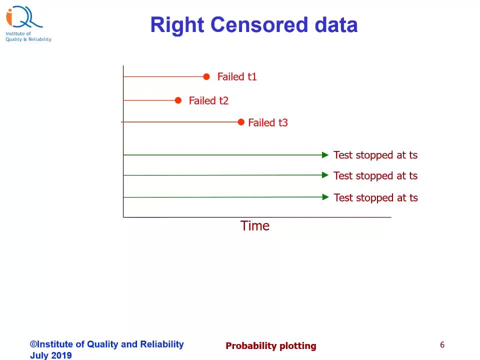 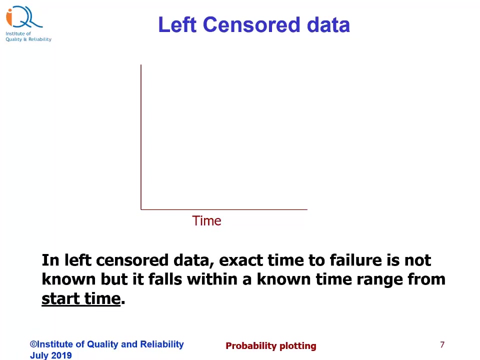 So all three component which completed the test without failure becomes right censored data And they have the same time, but we have stopped the test. Incidentally, this kind of testing is called time terminated test and the right censored or type 1 testing. Now we will look at left sensor data. In left sensor data: exact time. 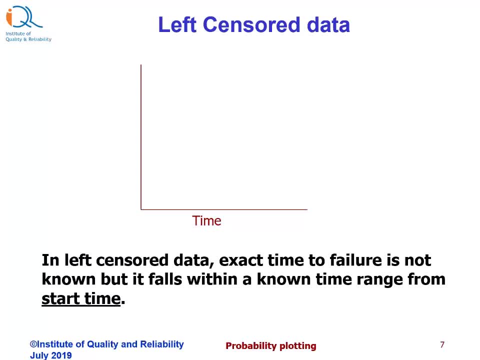 to failure is not known, but it falls within a known time range from start time. So, for example, a component has failed at a given time but we do not know when it exactly failed from the starting time. So there is an interval. second one also, it is a similar case. third, 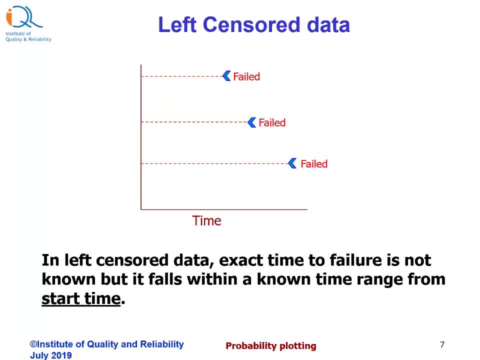 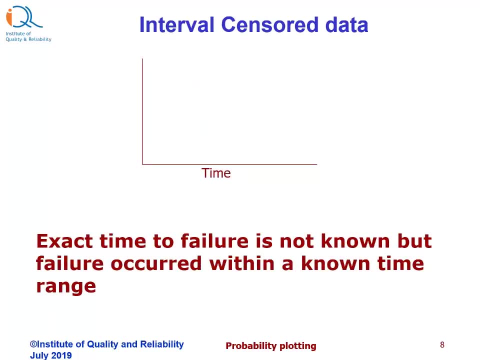 one also. it is a similar case, So this kind of data is left sensor data. Another type of data is interval sensor data. In this type of data exact time to failure is not known, but failure occurred within a known time range, For example in the first. 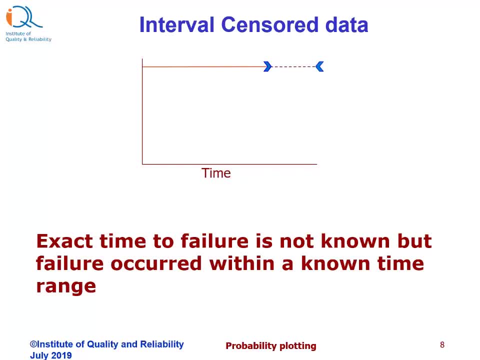 time. we know that it worked up to a certain time and later on we found that it failed. So we only know that it fails during a particular interval, but we do not exactly know when it failed. So this kind of data is interval sensor. It is very important to understand. 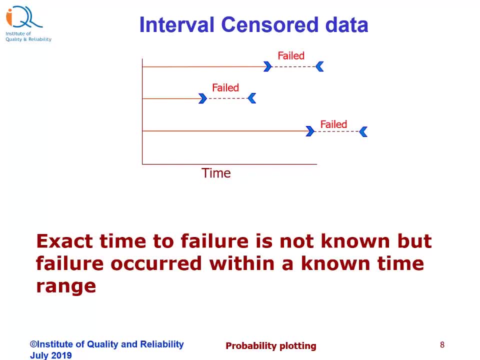 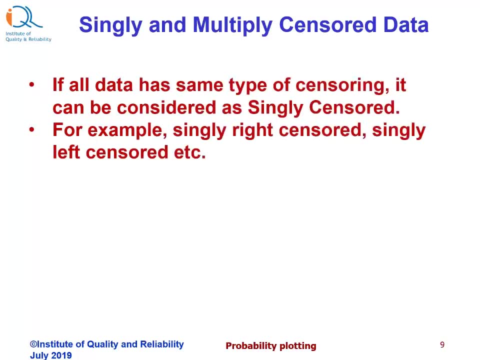 what kind of data we are analyzing. Accordingly, the procedure gets modified slightly. Let us understand singly and minimally multiply-sensor data. now, If all data has same type of censoring, it can be considered as singly-censored, For example, singly-right-censored or singly-left-. 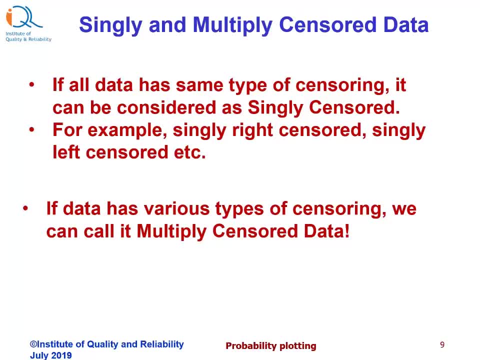 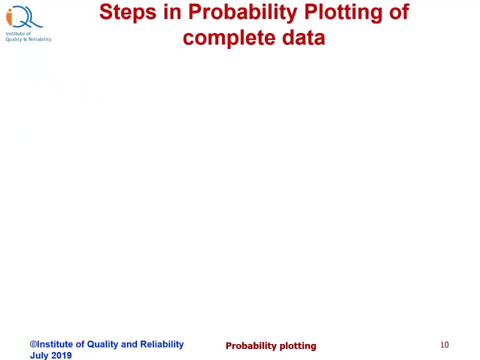 censored, etc. If data has various types of censoring, we will have to call it multiply-censored data. Let us understand steps in probability plotting of complete data. First, select data of failure times for a particular failure mode. Remember the weibull plotting or other. 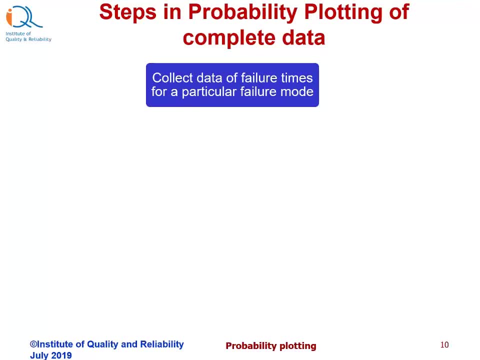 plotting of live data should be done for one particular failure mode at one point of time. If we mix different failure modes we may not be able to fit the data on a particular distribution. Next, arrange failure times in ascending or different situations. Calculate the median rank. We will learn how to do the median rank calculation and plot failure time versus median rank on a probability plot. 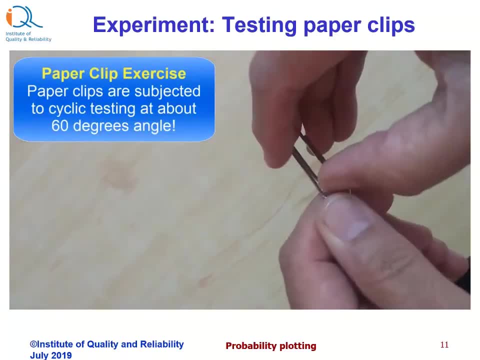 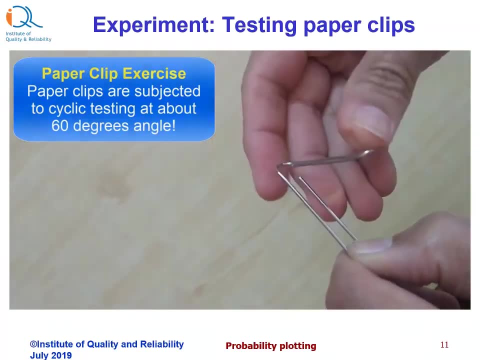 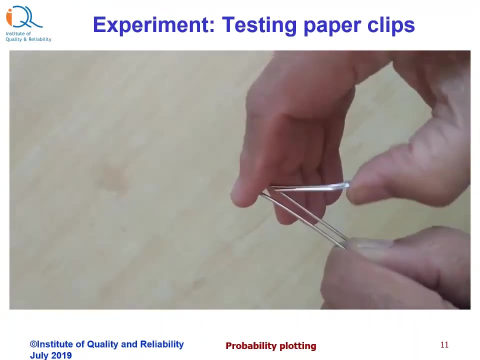 We will test some paper clips with 60 degrees open and close cycles. as you can see, Open, close, open, close. The 60 degrees angle is visually controlled to the extent possible. Now we will run the video clip fast to save time. 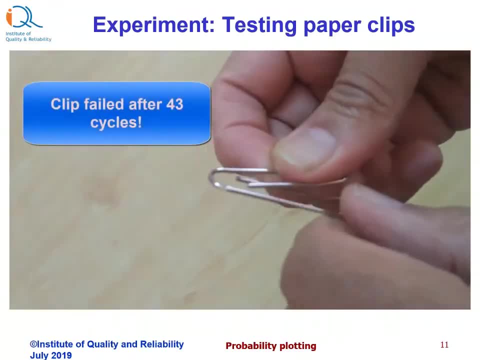 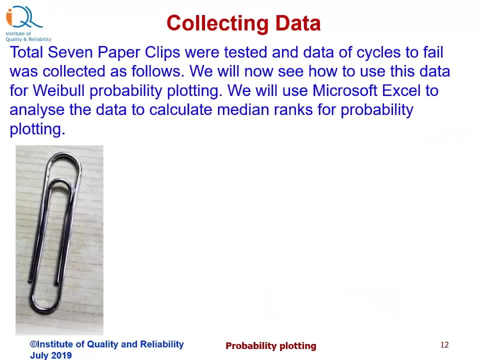 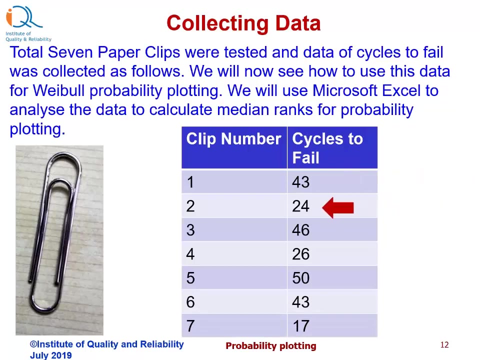 The paper clip failed at 43 cycles. as you can see, Total 7 paper clips were tested and data of failure times or cycles was collected, And this is the data: 43,, 24,, 46,, 26,, 15,, 43 and 17.. 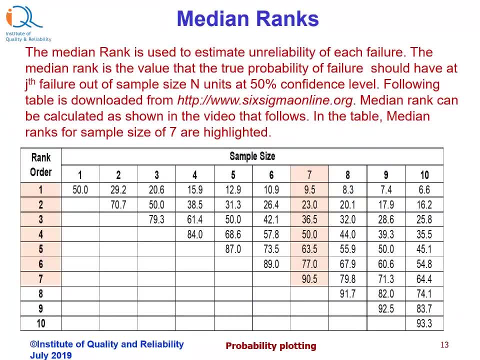 One of the important steps is to calculate the median rank. One of the important steps in variable probability plotting is calculation of median rank. The median rank is used to estimate unreliability of each failure. The median rank is the value that the true probability of failure should have at j failure out of sample size of n units at 50% confidence level. 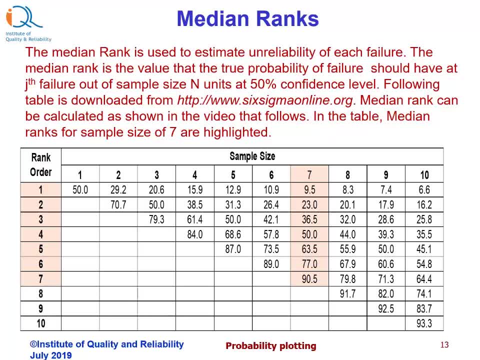 Following table is downloaded from the website 6sigmaonlineorg. Median rank can be calculated as shown in the video that follows. In the following table, the median ranks- of sample size 7 are highlighted. We will now use Microsoft Excel to process the data. 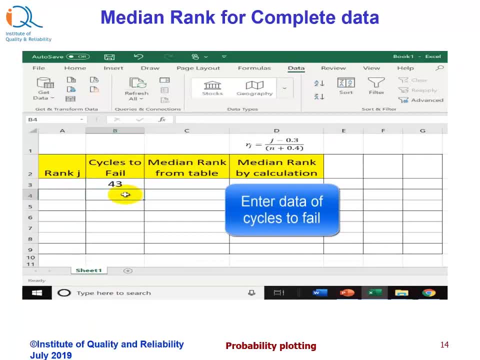 First enter the data of cycles to fail: 43,, 24,, 46,, 26,, 15,, 43 and 17.. After that we will sort the data of cycles to fail in ascending order. on Excel This is easy. 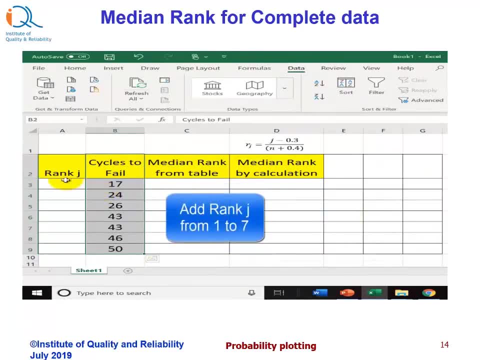 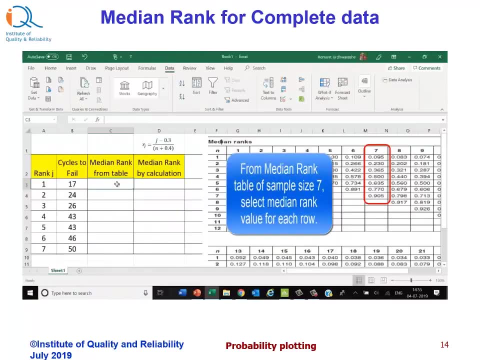 Then we give the rank numbers 1 to 7 to the 7 tested clips. Now we use the median rank table to estimate the median ranks of each failure, The first one being 0.095, 0.23, 0.265. 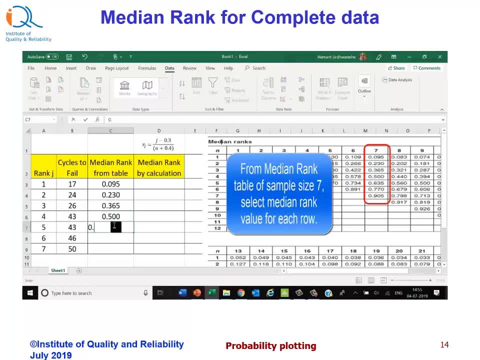 The median rank. tables are available for various sample sizes. We have marked the table for sample size 7 and using those numbers to estimate the median rank. Alternately, we can also calculate the median rank Rj by the formula shown: j minus 0.3 upon. 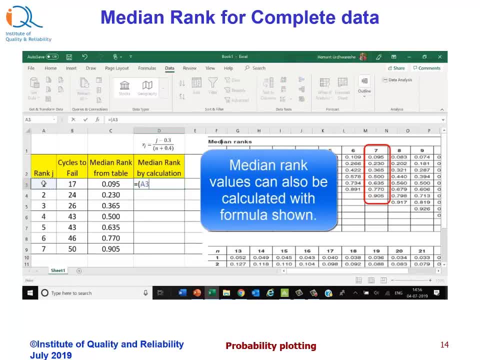 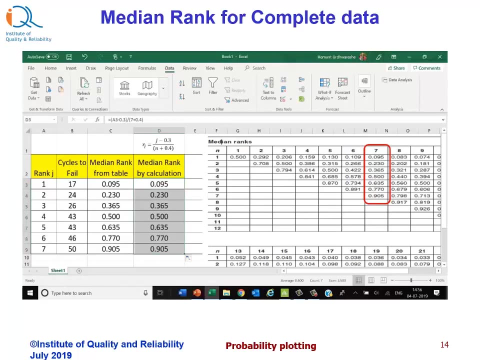 n plus 0.4.. So you can see the calculation on Microsoft Excel and you can also see that the values will match. So you can see the calculation on Microsoft Excel and you can also see that the values will match With the median rank table values. 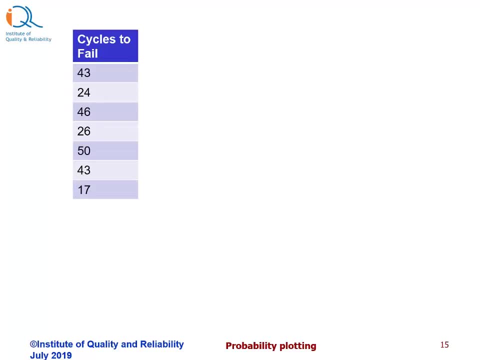 We have tested 7 paper clips and this is the data of cycles to fail for those 7 paper clips. Observe that the minimum value is 17 and maximum is 50 and therefore we can choose one cycle viable paper As these values are between 10 to 100, which is one cycle on a log scale. 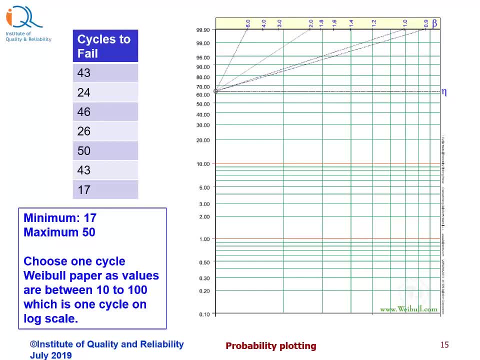 This is the one cycle log paper downloaded from website viablecom. You can get viable paper on many other websites. Mark the x-axis with cycles to fail from 10 to 100.. As you can see, the values are between 10 to 100.. 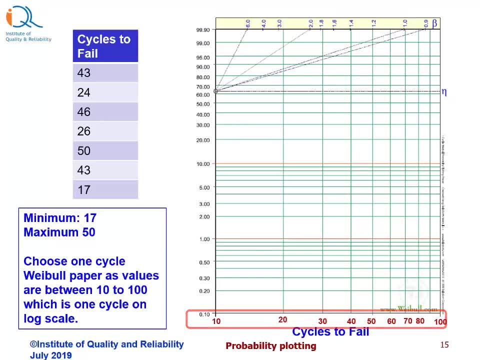 This is the one cycle log paper downloaded from website viablecom. You can get viable paper on many other websites. As you can see, the y-axis is already marked and we know that this represents the failure function, the cumulative failure function, and the cumulative failure function is capital. 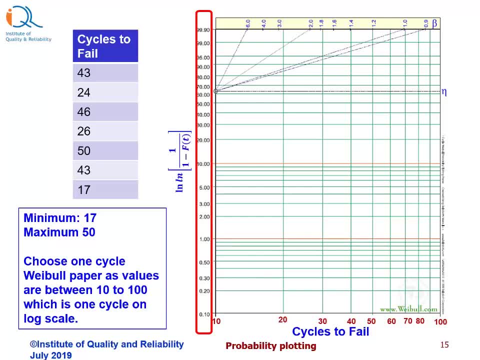 F of t and the function is ln of ln 1 upon 1 minus f of t. The top of the viable paper has markings to estimate the cycle. The top of the viable paper has markings to estimate the cycle. to estimate the shape parameter: beta. 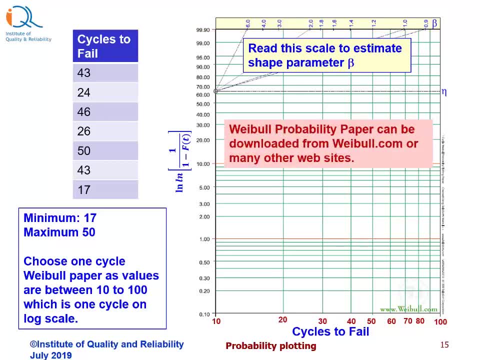 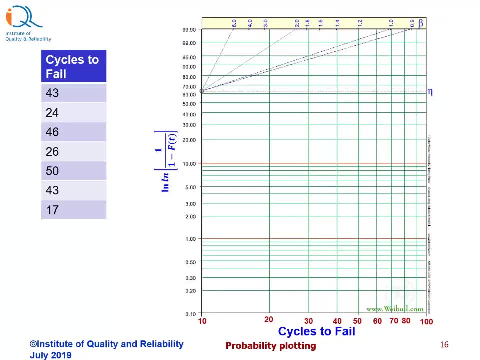 Weibull probability paper can be downloaded from weibullcom or many other websites. Now we see the Weibull probability paper with x-axis mark for the cycles to fail. We also see the data of cycles to fail for the seven paper clips. 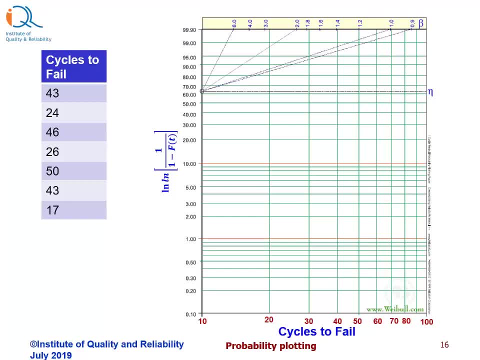 If we plot this data on the Weibull paper and if it follows a straight line, as can be seen in the video, we will conclude that the data reasonably fits Weibull distribution. Once we confirm that the data follows Weibull distribution. 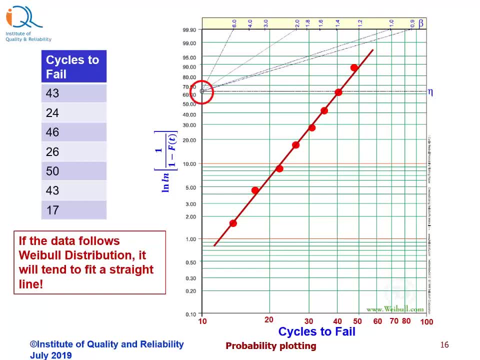 we can start estimating the parameters using the Weibull probability paper. First we estimate the shape parameter, beta. For that we draw a line parallel to the plotted line from the marked point as shown and read the beta parameter at the top of the Weibull paper markings. 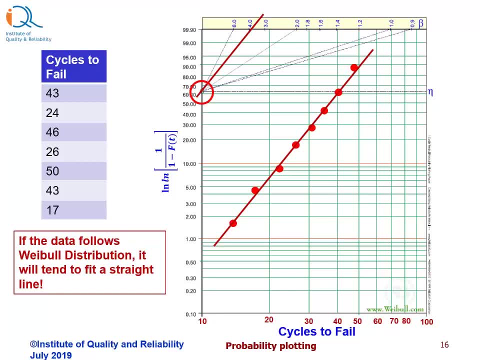 In this case it appears to be 3.9.. After this we try to estimate the scale parameter eta. The graph paper has got eta parameter marking at 63.2% failed parts. Now we identify a point of intersection between the plotted line and the eta line. 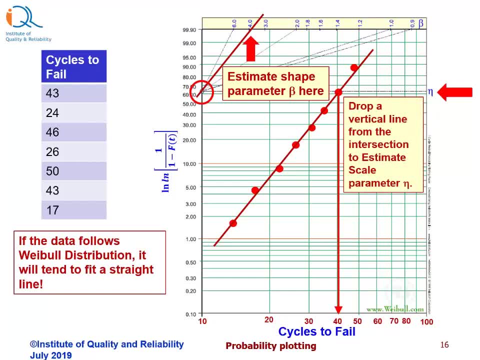 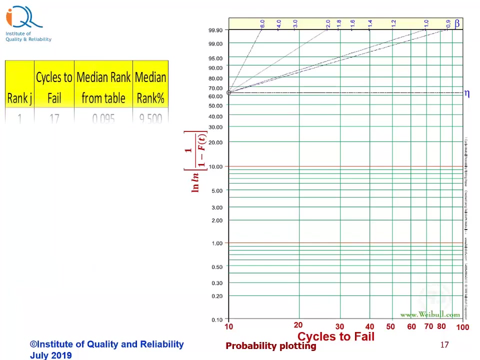 and draw a vertical line on the x-axis and read the eta parameter on the x-axis. In this case the eta parameter looks like something like 41.. Now we will see how to plot the data of cycles to fail of the paper cliff versus the median rank. 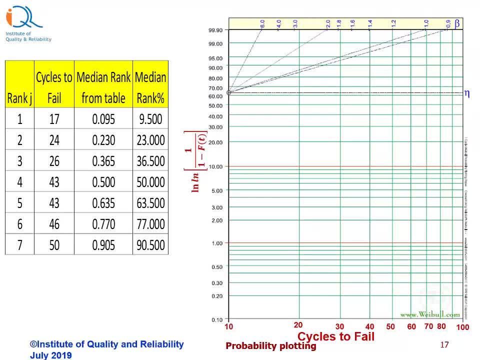 We have already calculated the median ranks, but we convert them into percent values by multiplying by 100, as our Weibull probability paper has got vertical markings of the percentages. So the first point: 17 cycles to fail and 0.095. will become 0.095.. So the first point: 17 cycles to fail and 0.095 will become 0.095.. So the first point: 17 cycles to fail and 0.095 will become 0.095.. 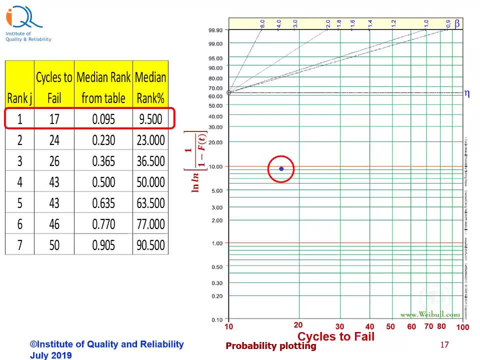 9.5 percent. So we plot that point. Similarly, the second point: 24 cycles to fail and 23.00% median rank. So we plot all the points and we can see that one of the points, that is the fourth point, somewhat does not follow the trend. 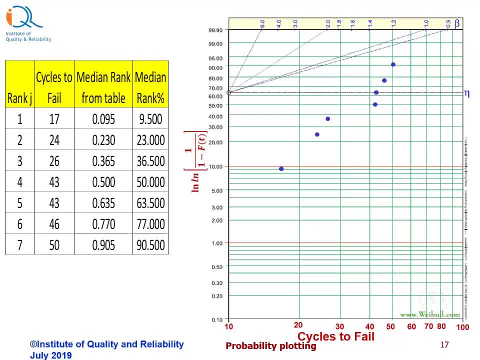 And we will have to probably check whether our data is correct or testing procedure was correct. So now we fit a line which appears to be the best fit line for the points plotted by dividing the equal number of points above and below. So this is the Weibull probability plot for the data of paper clips. 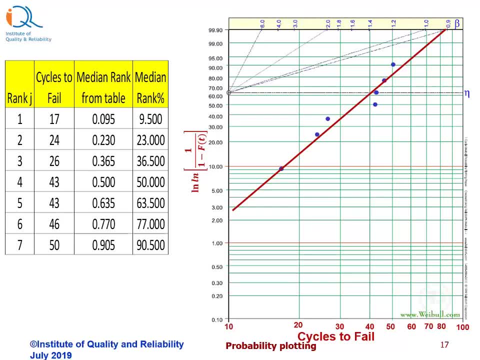 Now to identify the beta parameter or estimate the shape parameter. we draw a line parallel to the plotted line from the identified point and read the beta parameter on the top scale. Here the beta parameter appears to be about 2.8.. Now we have to estimate the scale parameter eta at 63.2 percent. 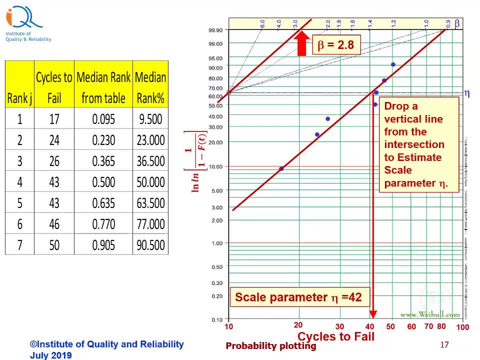 So we draw a perpendicular line from the intersection point and find that the scale parameter is about 43. We can also find out the beta in life by identifying the 10 percent point on the y-axis and then again finding out the point of intersection of this 10 percent horizontal line with the 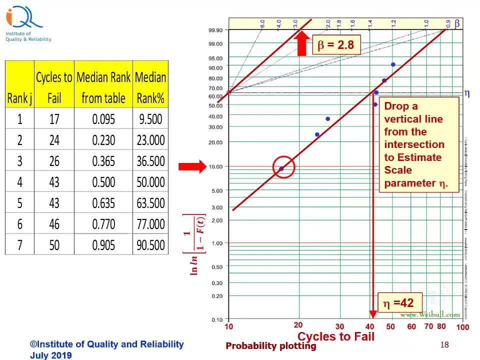 plotted line and again draw a vertical line from that intersection point to find out the beta in life. We can see from the graph that the beta in life is about 2.8.. And the beta in life is about 18 cycles or whatever. 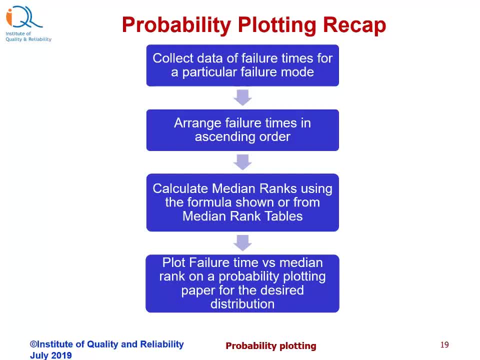 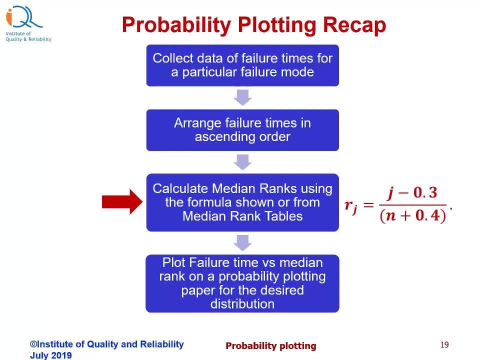 Then calculate median rank. Then calculate median rank using the formula shown or from the median rank tables And finally plot failure time versus median rank on a probability plotting paper for a desired distribution. In this case we have seen how to plot for a variable distribution. 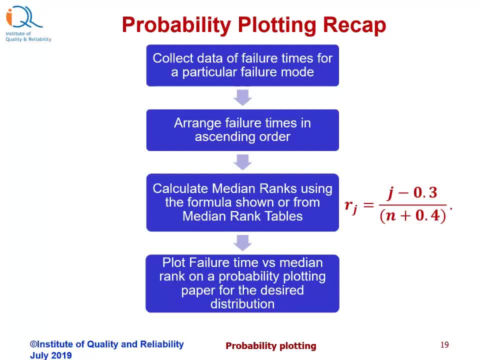 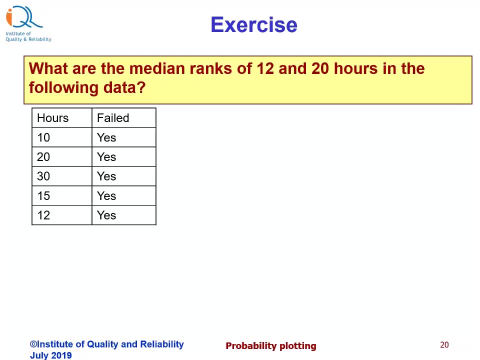 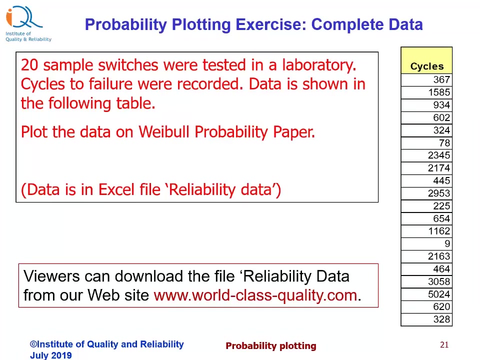 But probability papers are available for different distributions, such as normal, exponential log, normal, etc. Now you can try this exercise: Calculate the median rank of 12 and 20 hours in the following data. Another exercise: 20 sample switches were tested in a laboratory.